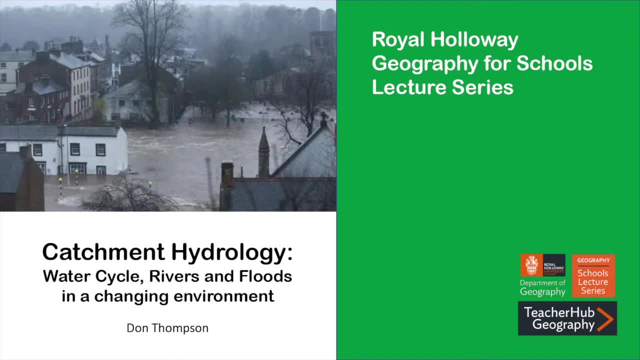 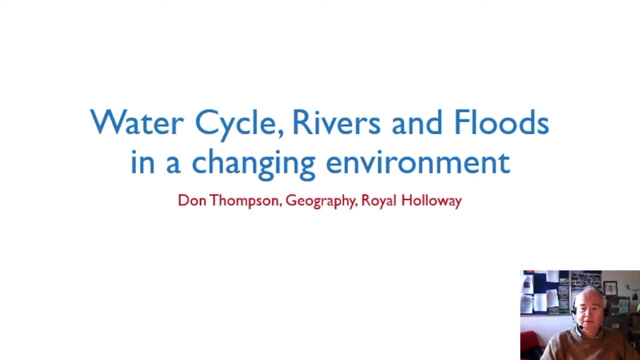 Hello and welcome to this talk entitled Water Cycle, Rivers and Floods in a Changing Environment. My name is Don Thompson. I'm Senior Lecturer in Physical Geography at Royal Holloway And in this talk I want to think about the ways in which human beings through land use. 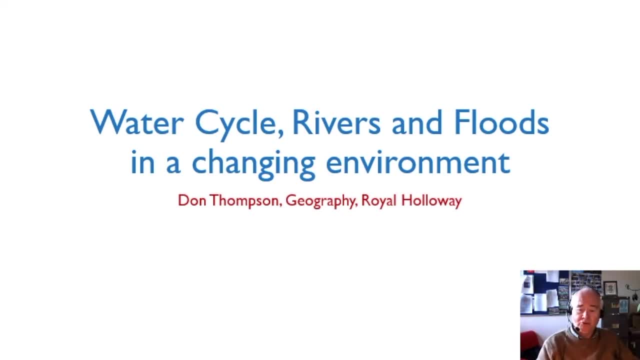 and through human-induced climate change, are leading us to think about different ways of managing flood hazard on our rivers. In the department I teach in year two on environmental processes and hazards and in year three on river management, And, of course, as we approach COP26,. 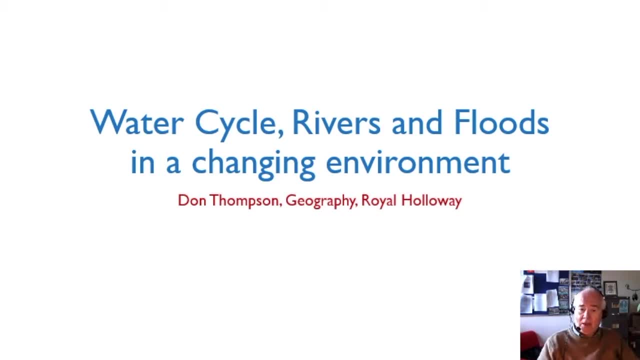 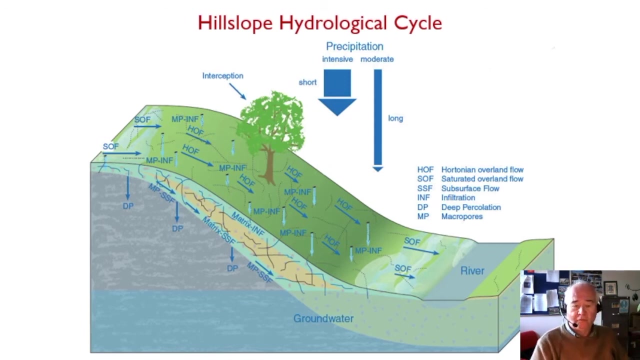 then. sustainability of environmental management is a really important issue facing the whole world, Not only restoring our climate and environment, but thinking about how we can manage the inevitable hazards in a more sustainable way, Fundamental to understanding the way in which flood hazard will evolve through the 21st century. 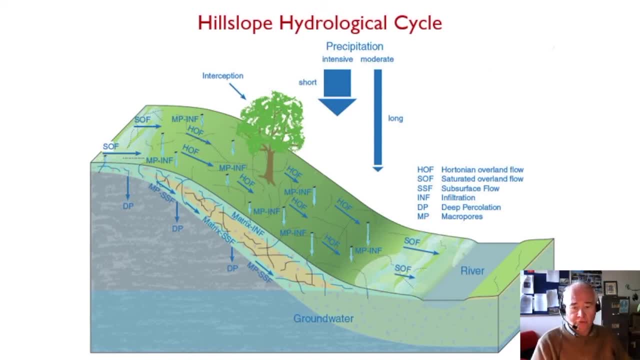 is our understanding of the hill-slope hydrological cycle, And there are two key elements that are relevant here in terms of global warming and environmental change. Firstly, climate: the amount, intensity and frequency of the precipitation falling on our climate. and that's coming back. 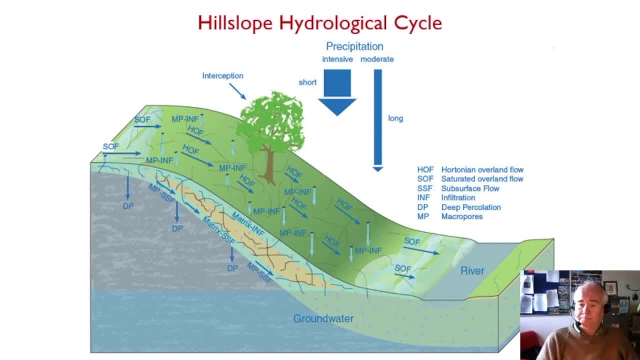 on our catchments is changing. The seasonality is changing. It's likely that we will have more rainfall in winter but less in summer. And then, of course, there's what happens to that rainfall, whether it percolates into the soil and runs through flow down to the. 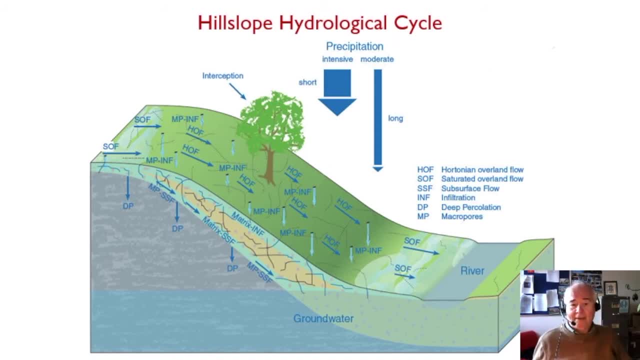 river through the soil, Whether it collects on the surface as Hortonian overland flow and runs into the river over the land surface, Whether the water gradually builds up and becomes saturated from beneath the soil and then ponds on the surface and runs over into the rivers as saturated overland flow. All of those routes are the. 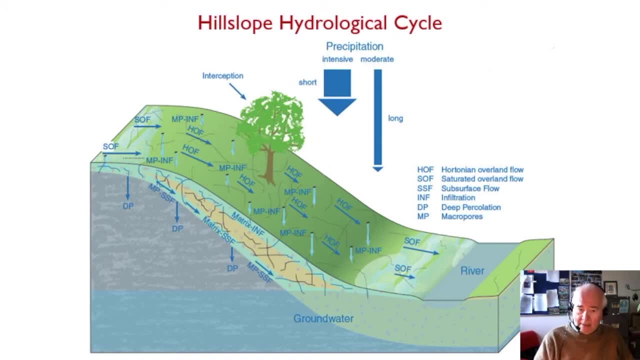 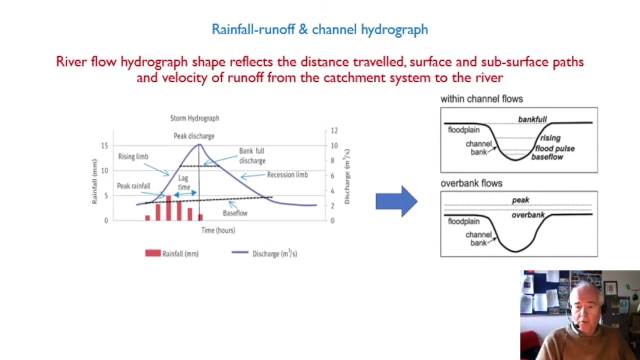 way in which we have impacts on the surface of the landscape and on our soils and on our vegetation cover will affect that relationship between what happens in the catchment and what happens in the rivers. The output of runoff from the hillslope hydrological cycle from the river catchment. 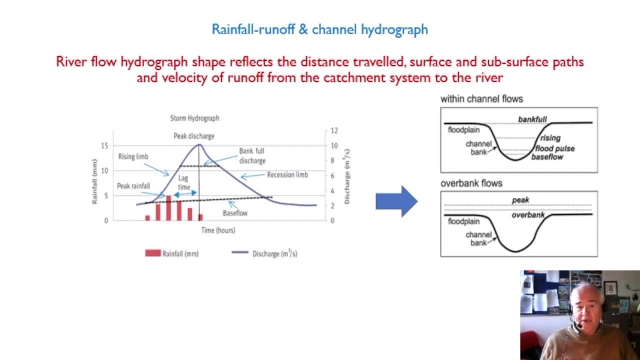 is measured in the river channel as the change in the flow of water. The change in the flow of water elsewhere is known as a rule of Lane change in flow discharge over time And this is called the flood College Geograph, And it will have a lag behind the input of rainfall. 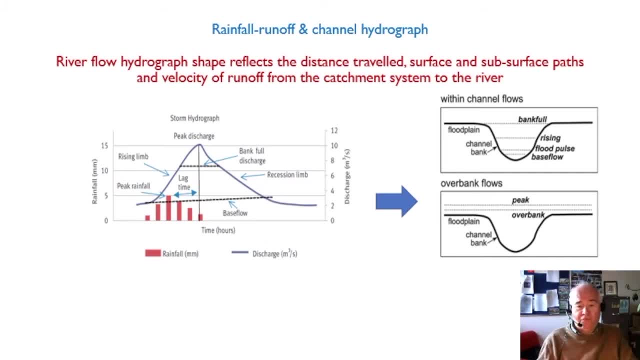 Because the water needs time to flow from the slopes, either over the surface or you the soil, to reach the river channel. in response to a rainstorm, The flow of the river will increase and it may attain bankfull. If the flow continues to rise to a peak discharge that is over bankfull, we have the definition of a flood. 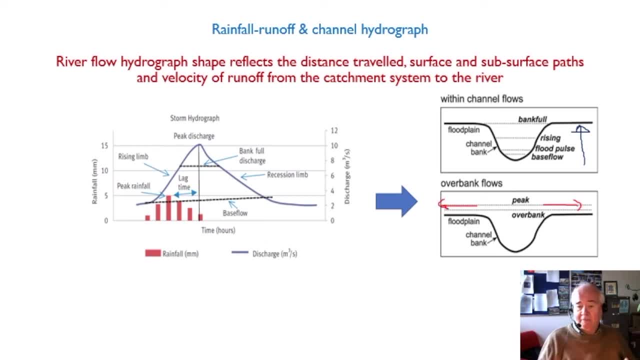 River discharge that exceeds bankfull And then the river floodplain is inundated with water and the floodplain stores that flood water. That's the essential mechanism of flooding. The question we're thinking about in the 21st century is whether the frequency and the severity of that flooding 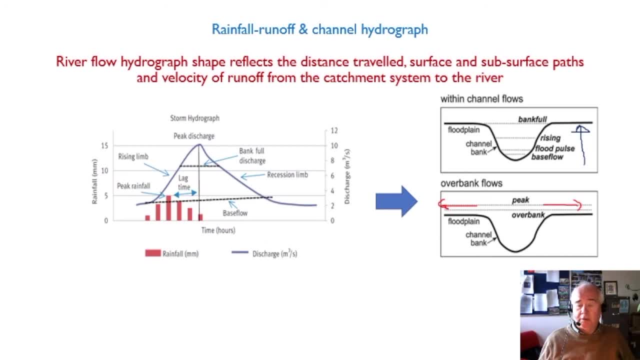 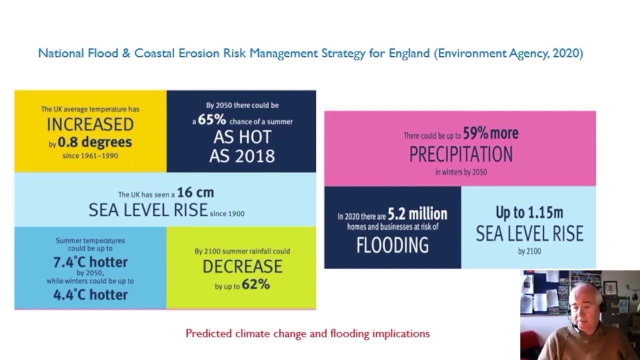 will respond to environmental change, and environmental change In particular to climate impacts. We know that the peak rainfall is likely to increase in winter and that rainfall intensities may increase in summer even if the totals are reduced. The National Flood and Coastal Erosion Risk Management Strategy for England, published last year by the Environment Agency. 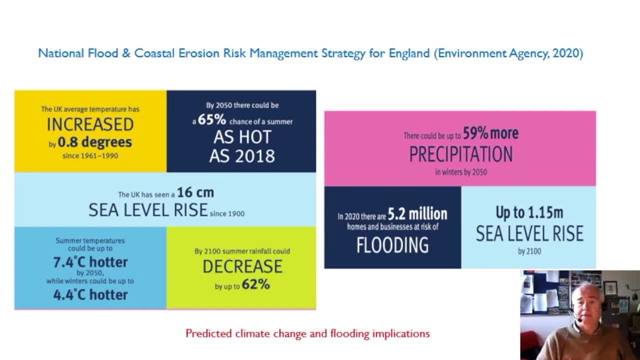 gives us a context for thinking about these hydrological cycle and flooding issues in the 21st century. We know that between 1961 and 1990, average temperature increased by about 0.8 degrees, But we know that by 2050, summers could be up to 7.4 degrees centigrade hotter. But we know that by 2050, summers could be up to 7.4 degrees centigrade hotter. We know that by 2050, summers could be up to 7.4 degrees centigrade hotter And winters could be up to 4.4 degrees centigrade warmer. The chances of extreme weather, such as extreme heat or extreme rainfall, are likely to increase through the century. So by 2050, we could have a 65% chance of a summer as hot as that of three years ago. We have already had 16cm of sea level rise since the beginning of the 20th century. By 2100,. summer rainfall could decrease by up to 62% By 2050,. there could be a decrease in precipitation in almost two thirds of winter By 2000,. there could be little more increase in precipitation in winter Until the spring of 2050. 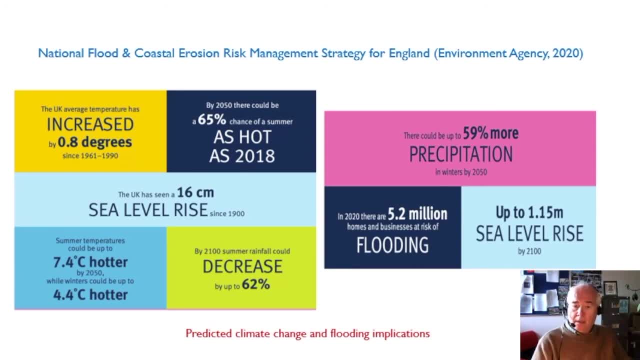 In 20 guiding clouds, there could be flow permitting higher TTR and greater QSHR returns To go beyond that risk of 0.9 degrees centigrade, over 20.17 degrees centigrade In 2020, there were 5.2 million homes and businesses at risk of flooding. 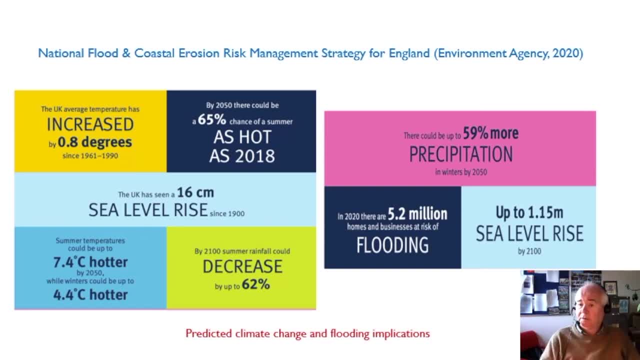 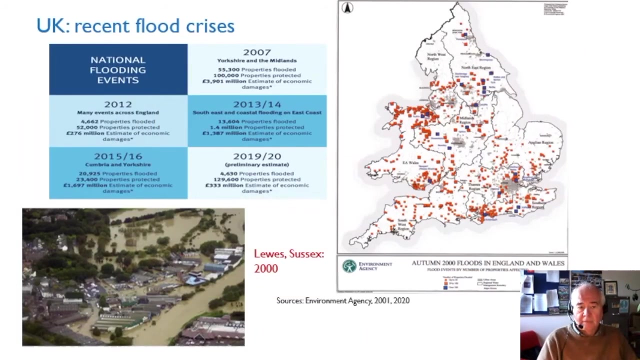 and by 2100 sea levels could have risen by over a meter under some of the global warming scenarios. So the context for the flood hydrology of Britain could be changing very significantly In the next few slides. I'm just going to go through some of the significant 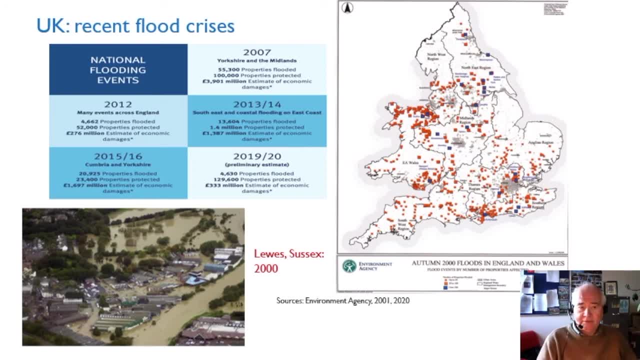 flood emergencies that we've had in the 21st century. We seem to be going through a flood-rich period in northwestern Europe and in the UK more generally, with several key flood emergencies having occurred since the turn of the century. In the year 2000 there was major flooding across England and Wales. some of the 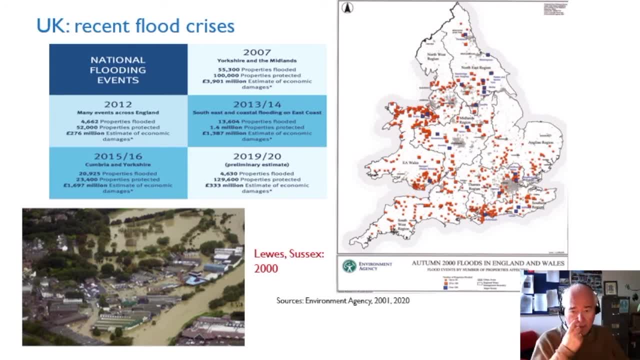 most widespread flooding in the recent history of the UK. That occurred during the autumn, particularly in October and November. It flooded places such as Lewis, Newcastle and Leicestershire and from the map you can see the extent of damage to housing and the number of properties affected. In 2007, there was severe flooding in the summer. 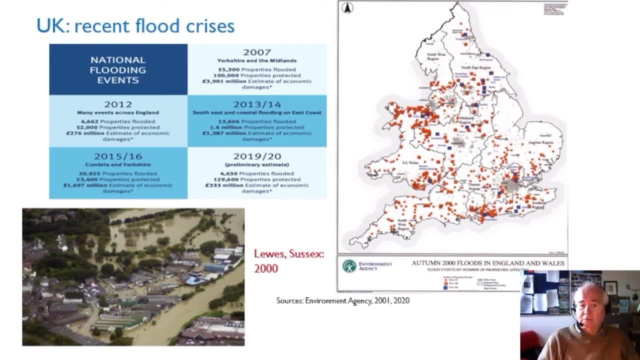 June and July in Yorkshire and the Midlands Over 50,000 properties flooded and in that particular year, nearly four billion in the economic sector was also damaged. We have experienced a significant level of damage: four billion pounds of damage to the economy. That involved the flooding of electricity substations and it revealed the threat to 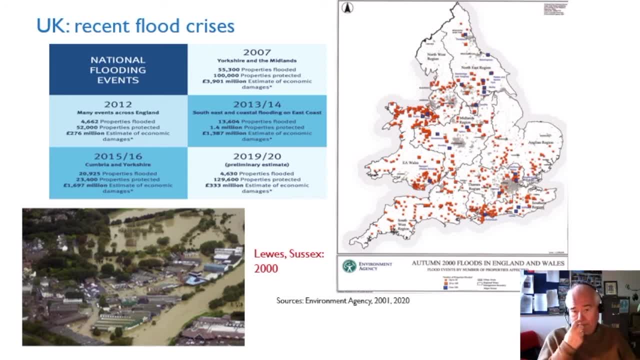 emergency services such as electricity, water and also access to hospitals. that can occur when you have a flood emergency 2012,. again a very wet summer with over 4,600 properties flooded, 276 million in estimated economic damage. Then really severe weather through the winter of 2013-14, over 13,000. 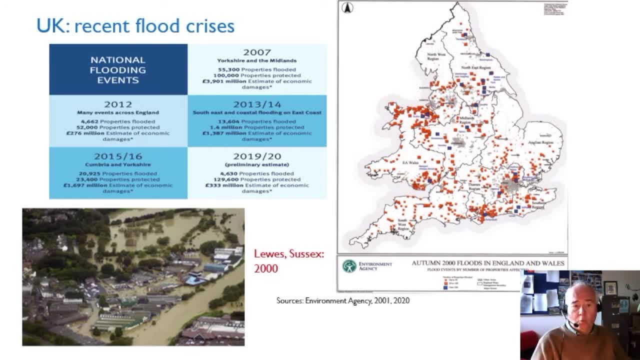 properties flooded and 1.4 billion in damages 2015-16,. 20,000 properties flooded, 1.7 billion in damages And a series of three severe storms causing localised flooding and hundreds of millions of pounds worth of damage in 2019-20.. 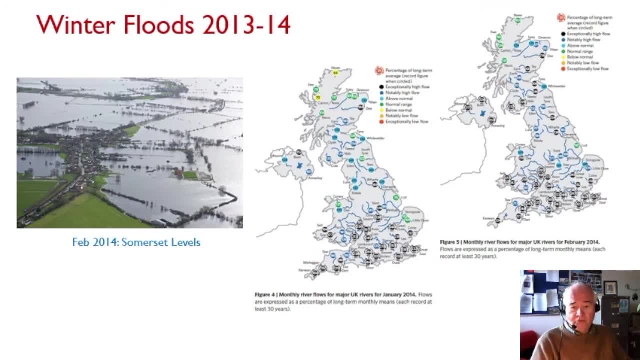 Just to pick out a bit more detail on the characteristics of some of these emergencies: in the winter of 2013-14, we had a series of extremely intense storms tracking across the Atlantic Ocean towards Britain. These were triggered by extreme cold in North America. 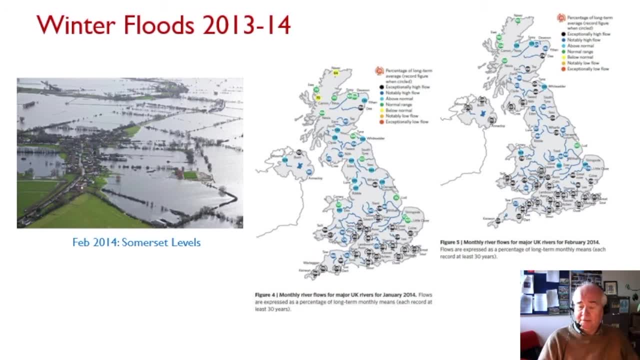 which contrasted with the extreme cold in the United States. The weather in the mid-winter period was also contrasted with the tropics- the warmth of the tropics to generate an incredibly strong Atlantic jet stream which drove intense storms straight into the path of the UK. The figures in the maps on this slide show the 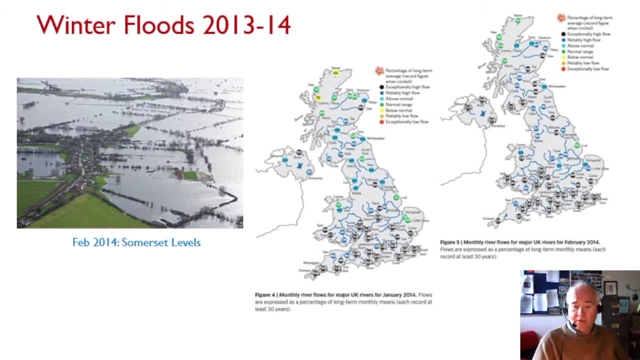 data for monthly river flows for major UK rivers in January and February of 2014.. The above Figures there of 250 to 300 percent of normal flows across much of southern England and in February extending up into northern England, Scotland and Northern Ireland. This was the year 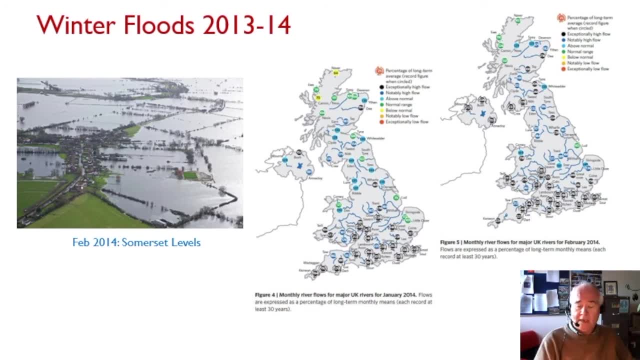 when the rail link to Cornwall was cut by severe wave damage produced by gale force winds tracking across the Atlantic. It was a year when the Somerset levels were flooded for nearly two months in some locations due to the severe river flooding. Just two years later, the focus moved. 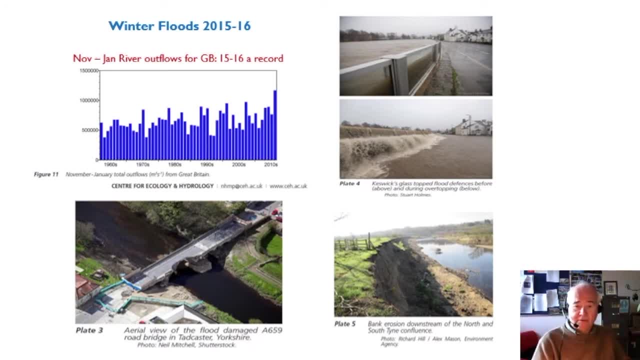 more to the north, with a series of storms producing severe flooding in the Pennines, Yorkshire and northern England. The November to January river outflows for the country as a whole reached a peak in the winter of 2015 and 16.. The characteristics of these floods were somewhat 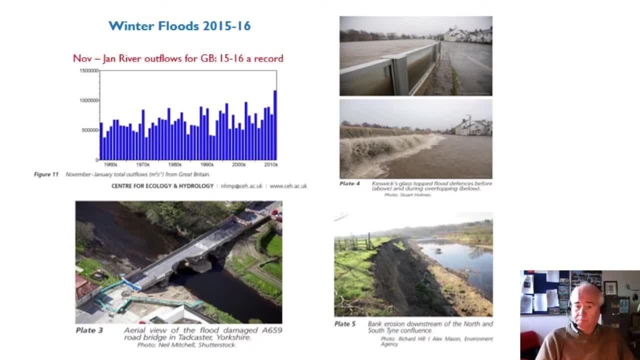 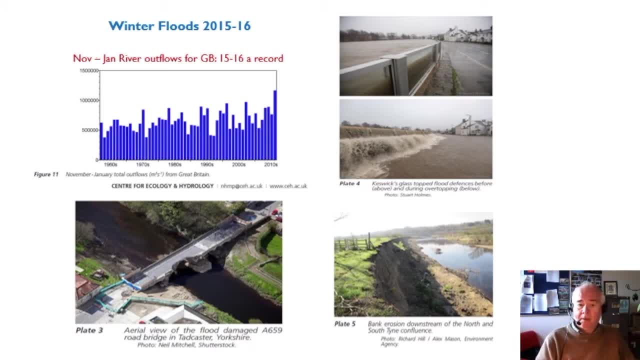 We can see the picture of the flood defences in the Lake District town of Cornwall. The two lower photographs show that the characteristics of these floods wasn't just inundation of houses by water. it was also severe erosion and mechanical damage to infrastructure. The flood dam was cut off from the 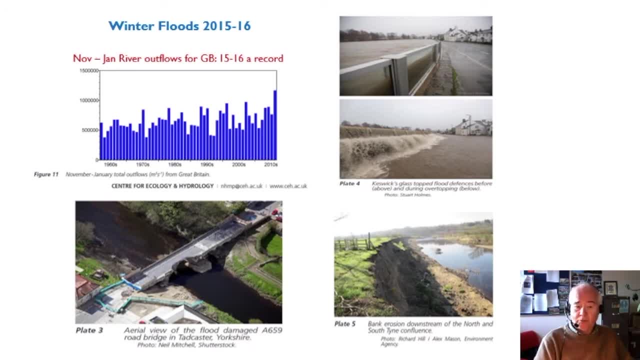 other, by the severe damage to the bridge. This was the episode of the flood dam in Cornwall and the bridge, which meant that the journey to get your newspaper from one end of town to the other could take an hour, because you had to drive all the way around the roads to find. 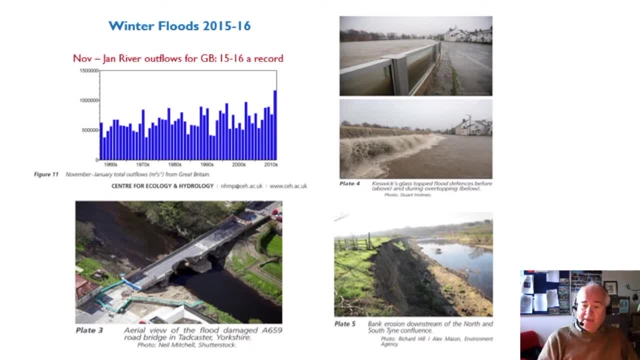 a route to the other side of town. Severe erosion occurred on rivers, such as a bank erosion on the Tyne River in Northumbria, and this was because the floods were hitting upland catchments so that the flood in the rivers was generated, had very high velocities and very high 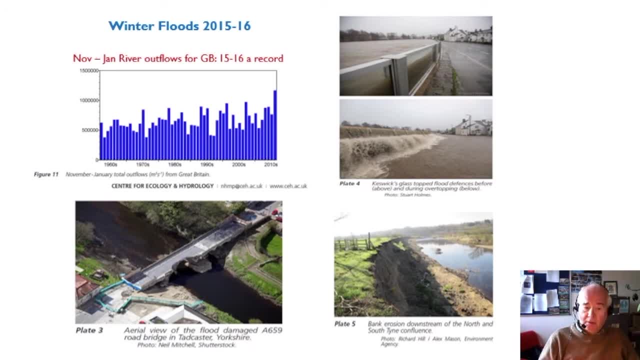 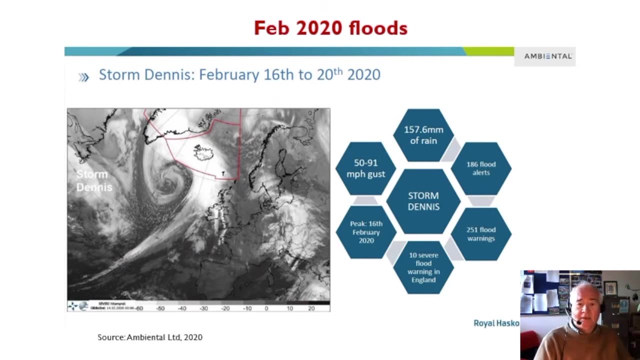 energy that led to mechanical damage to structures and severe erosion in a way that wasn't seen in the more lowland river floods of two years before. In 2020, a series of three major storms tracked across the UK, bringing more localised but still severe and repeat flooding in parts of 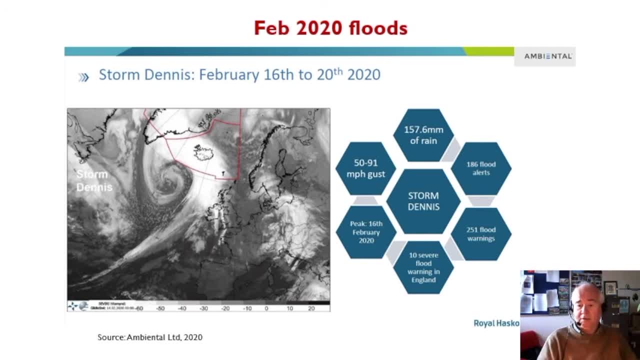 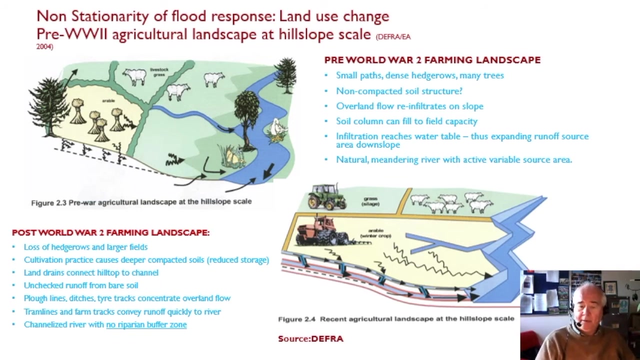 northern England. Storm Dennis was an example of that, with up to 91 mile an hour gusts of wind and nearly 160 millimetres of rainfall, producing 186 flood alerts and 10 severe flood warnings in England. So we've seen that we appear to be in a period of disturbed weather conditions. 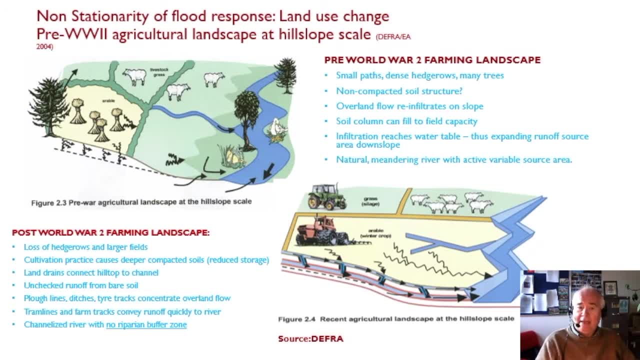 with frequent extreme rainfalls and very powerful storm systems. We have had some periods like this before, so the recent wave that happened in the flood rich period in the late 1900s and into this current century is not necessarily unique, but what we can say is that this increased storm. 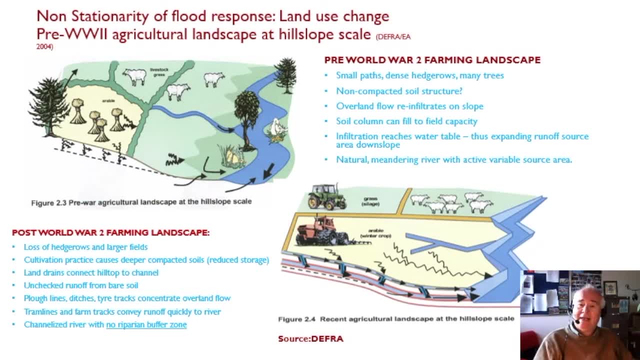 activity. an increased flood frequency is not inconsistent with what we would expect in an energised atmosphere, pretty much the same as rain can be seen anywhere. e ashamed we want to two produced by global warming associated with human greenhouse gas emissions. but of course, the storms and the rainfall is only one half of the picture. 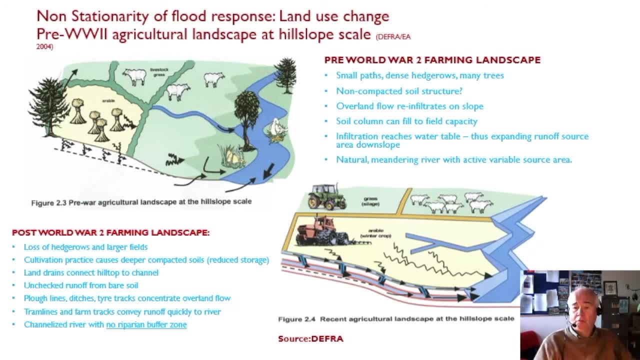 the other half is the landscape on which that rainfall uh falls, and we need to think in, if we're thinking about the hydrological cycle, about the nature of the land surface, the soils, the vegetation cover and the way in which human beings manage the landscape. if we look at just one aspect of this, the 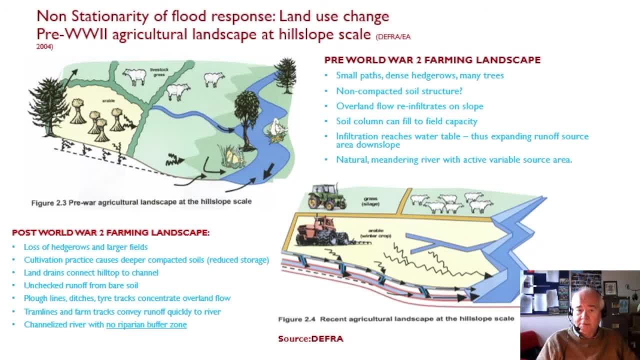 land use in our rural environments in britain in two periods, pre and post world war ii, we can see how things have changed massively. so before world war ii, generally fields were small. livestock numbers were low. each field was bounded by a hedgerow. cultivation generally only occurred for crops in the summer. 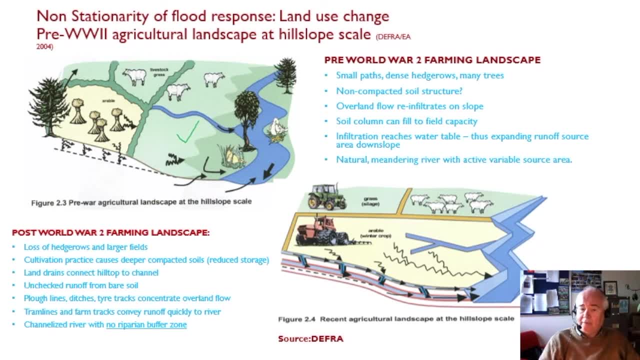 there was a greater tree cover. the banks and the boundaries of our rivers were generally well vegetated and not degraded. the rivers themselves were natural in terms of their meandering habit and a lack of human intervention in the boundary and the nature of the river channel. the soils were tilled through natural methods, without heavy combine harvesters or tractors. 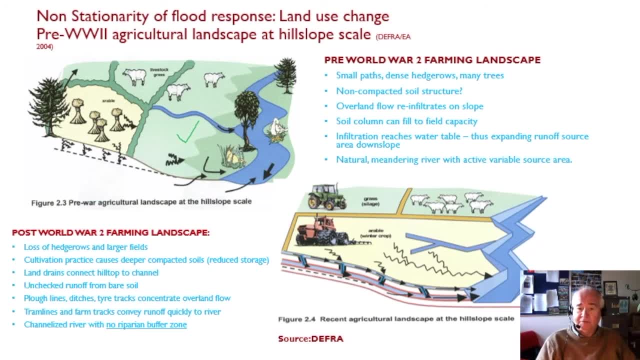 and that meant that the ability of the soil to absorb rainfall was greater. its infiltration capacity was greater than we see normally. Fukui and Taddei: across the pond tutteumahhara, lots of structures on thehyun ground. they were not in fact whatsoever traits. hetero: Willie therament of the south of mysterious f France. as i said, we see officials. 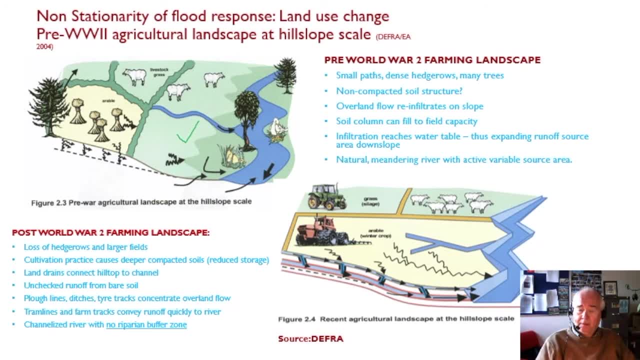 greater than we see more recently. contrast that with the post-world war to landscape. the war itself, triggering the need to grow more food, led to the start of cultivation the whole year round. winter crops bringing more land into production, increasing with field sizes, cutting down the hedgerows, intense cultivation, very large farm machinery that's efficient but compacts the soil. 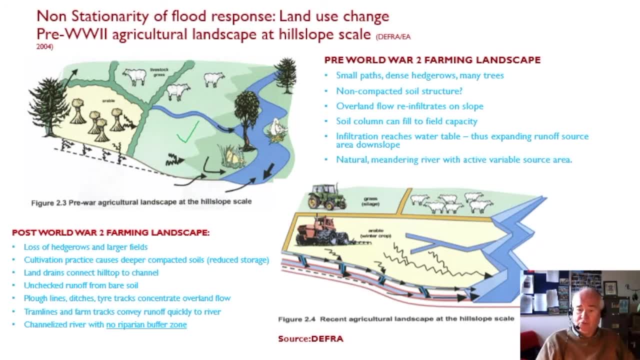 large field sizes, the removal of those hedgerows, the increase in the numbers of sheep, cattle and other livestock, compacting the soil, the installation of under soil drainage to improve the quality of the arable soils for winter crops and to prevent water logging. okay, all of these. 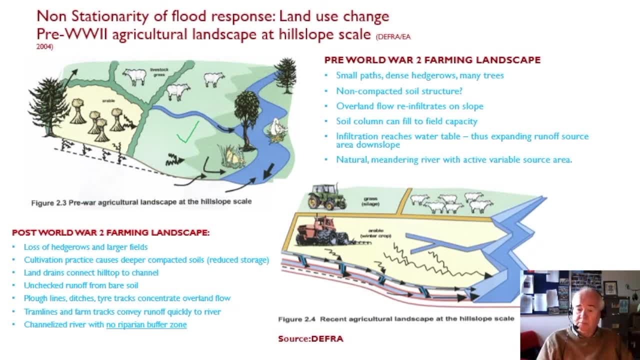 increase the link into hydrological terms between the farmland and the rivers, the rivers, themselves engineered to reduce flooding, straightened with artificial banks. the trees and the hedges from the rivers have started to drain down on the rivers, and so they've been continuing to help them grow from éjection. bạn overboo upoo, we can look. 살�, 하지만 vw. 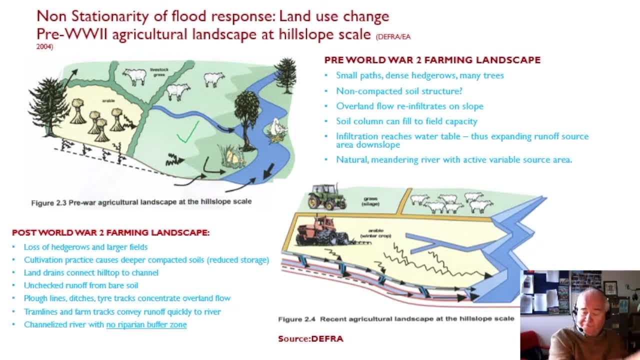 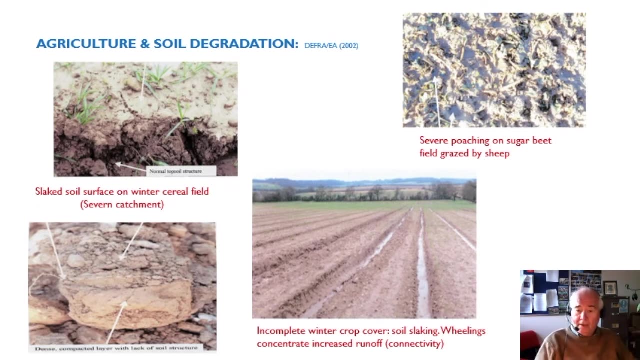 millennial iye. we can see some examples here of the way in which farm evolution has increased the connectivity of the landscape to the river. it means more runoff, compacted soils due to vehicles and due to livestock- what we call poaching, that is, the hooves of sheep and cattle. 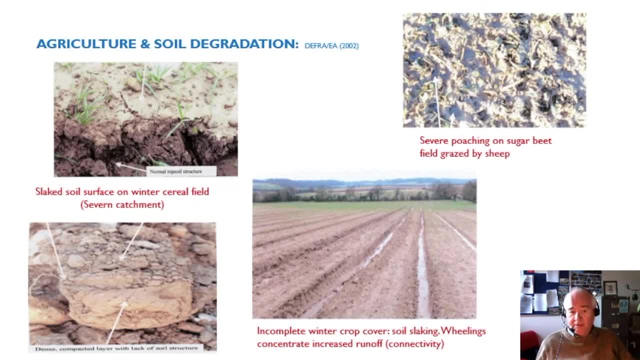 compacting the soil surface, producing subsurface compaction. that means that the rainfall can't filter down slowly into the soil but it tends to pond on the soil surface and run off wheelings produced by farm vehicles, often during the seed planting process. okay, leading to the channelization of 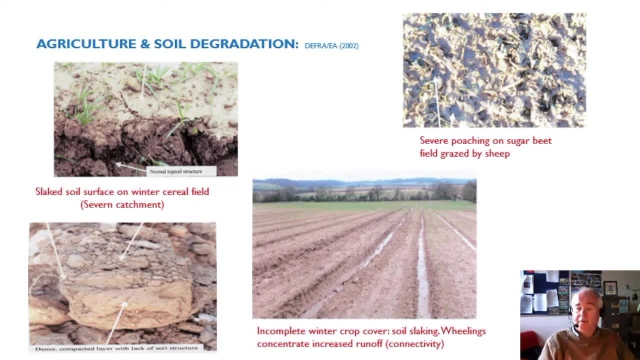 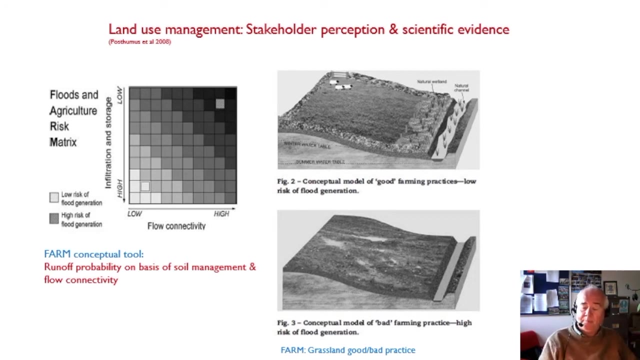 water and the accumulation of that runoff in large fields, no longer held back by ditches and hedgerows, before it gets to the river. all of these issues have led to a farming landscape in which two things happen. firstly, risk of runoff is increased because the infiltration rates of the soil are generally lower than they used to be. 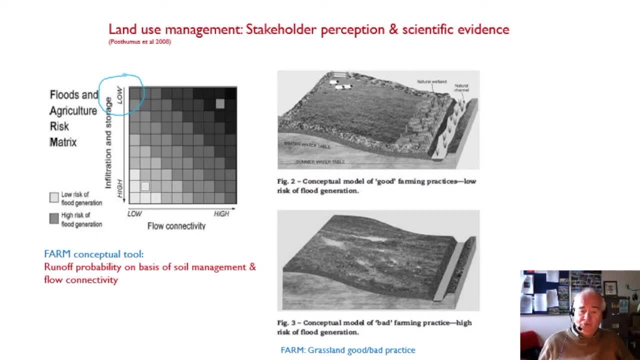 and secondly, the removal of hedgerows, the use of large farm machinery, increasing the connectivity between the fields and the rivers. the combination of these two things produces high risks from agricultural lands use, high risks of flood generation. so what do we need to do about our land use? well, we need to think. 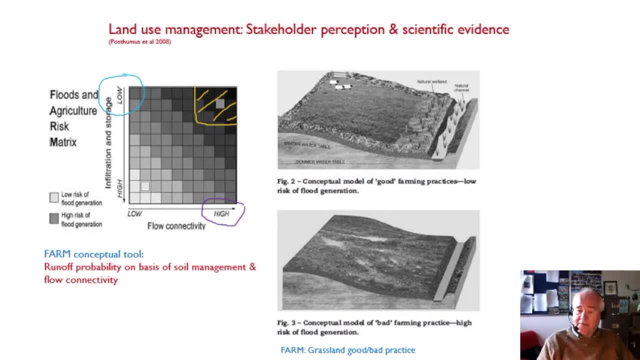 about farming practices that reduce runoff generation and reduce connectivity between the fields and the rivers, and work such as that by posthumous et al, as illustrated on this slide: work with farmers to help to talk to them about the way in which they perceive flooding, what damage it does to 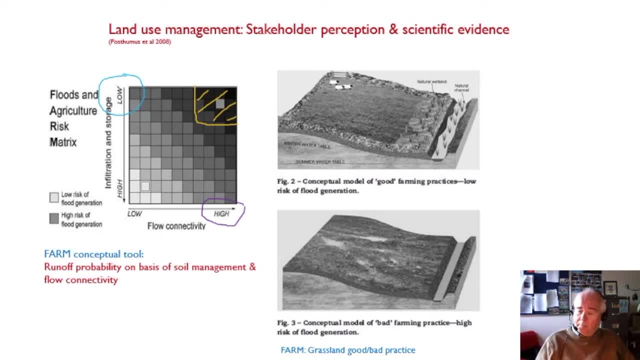 their own livelihoods and how they can adapt their farming practices to reduce the generation of floods from their landscape. all of this is good practice now and is happening, and that's positive. but we have a long way to go, given the changes that have occurred over the last century and of 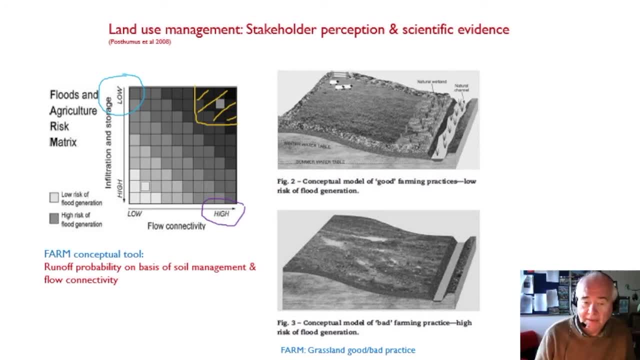 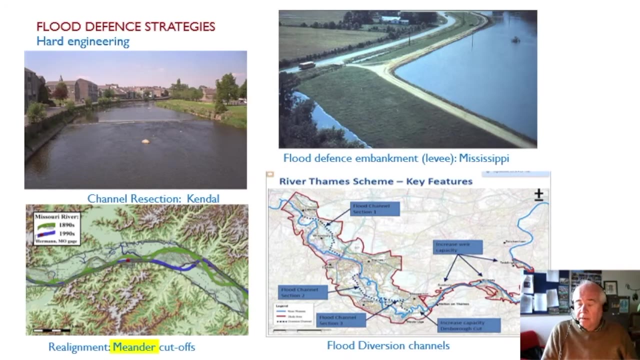 course that's just the farmland. we're urbanizing our catchments very rapidly: population growth and urbanization building on the floodplain. what can we do to reduce the generation of floodplains? about that, of course, flooding has always happened and we have always needed to protect populations. 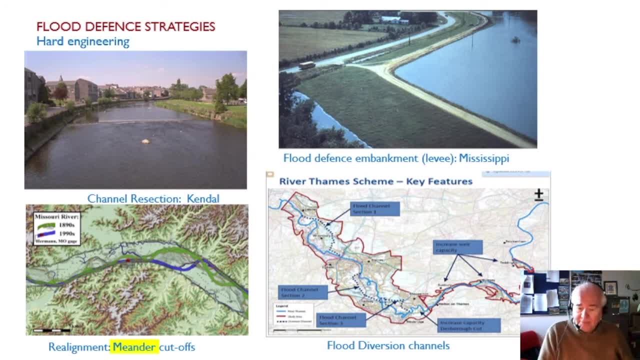 towns and our landscape against the hazards associated with flooding- hazards to life and hazards to economic activity. traditionally in the much of the the 20th century, the approaches to flood protection have been through hard defenses. for example, we can see here what we call channel resection: making the river channels in our urban. 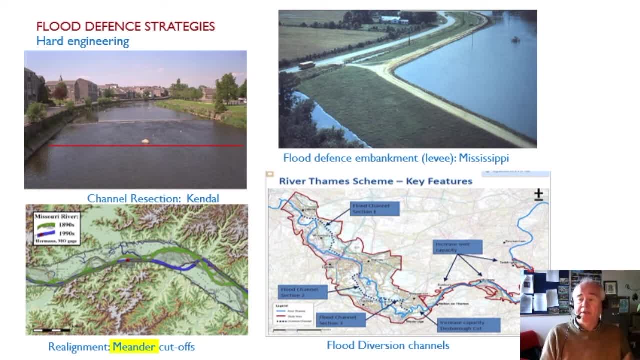 areas bigger in order to be able to contain flood water so that it doesn't flood the town. that has a major impact on the ecology of the river, of course, and can lead to a whole range of of issues unrelated to the flood protection function but which perhaps we might see as negative in terms of sustainability. 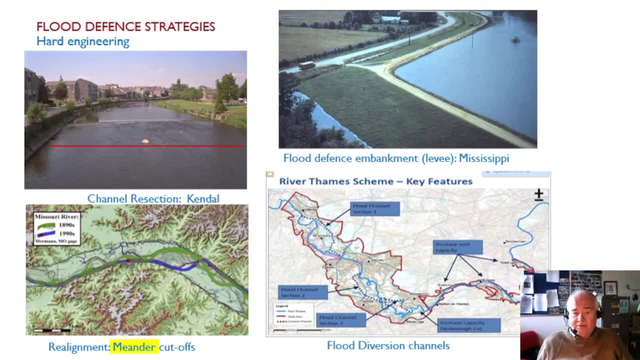 we have cut meanders off, we've made the river less bendy and we've made it straighter to make the water flow more efficient and therefore to reduce the chances of the water spilling over onto the floodplain. examples there, particularly in some of the major rivers of the world, such as the Missouri and the Mississippi in. 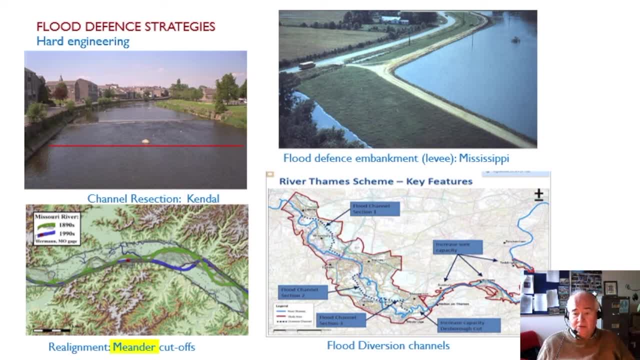 the USA we've raised the banks of our rivers to form levees to protect the surrounding floodplain, so that we can build on it, so that we can cultivate it. but of course the danger of a levee bursting then threatens potentially more severe flooding. but there's no doubt that hard defenses have allowed human flourishing and economic. 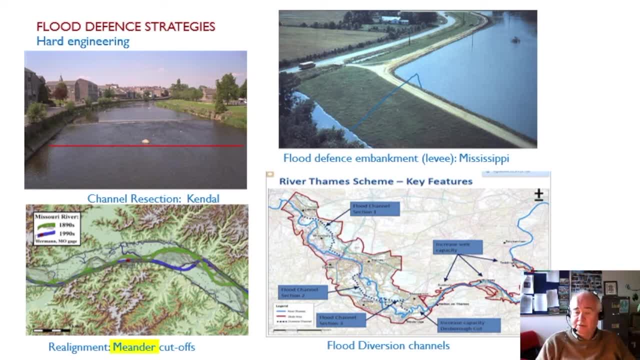 development. the question is: are they always the most effective ways to protect against flooding, and are they the best ways to go forward into a century in which flooding may become more severe or more frequent? more locally, near to Royal Holloway, we have the example of a major, hard engineering projects which 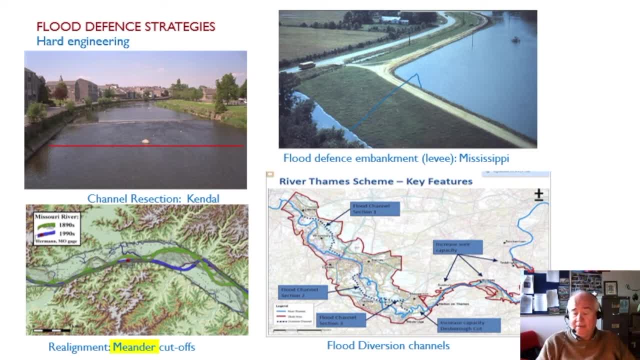 uh have been done in this century and are, which are, which are planned further for the next 10 years, and that's the use of flood diversion. and that's the use of flood diversion on the Thames, building additional stretches of river channel that connect parts of the Thames course. 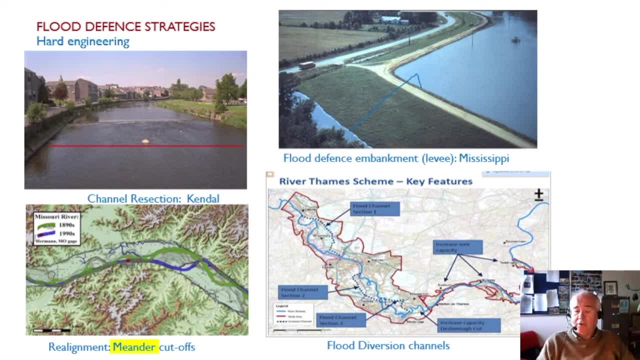 so that water can be diverted into those channels when a flood is threatened, protecting currently areas like Windsor and Maidenhead but planned channels likely to be um implemented to protect the Egham area and further downstream towards waybridge and water non-thames. so hard defenses have been the first choice for flood Defense. they've been really successful. 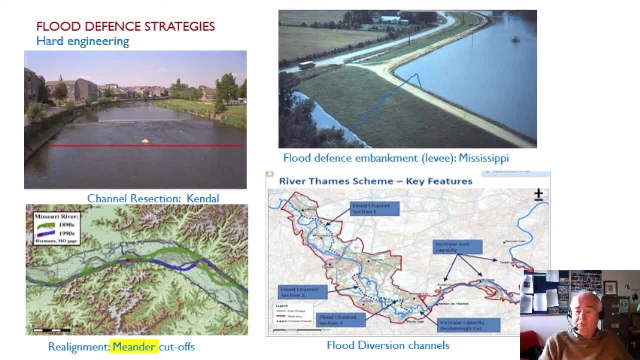 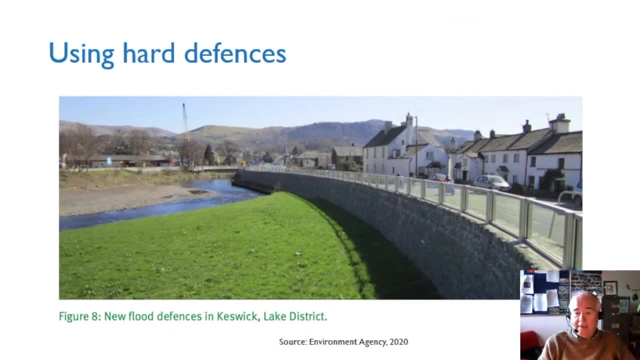 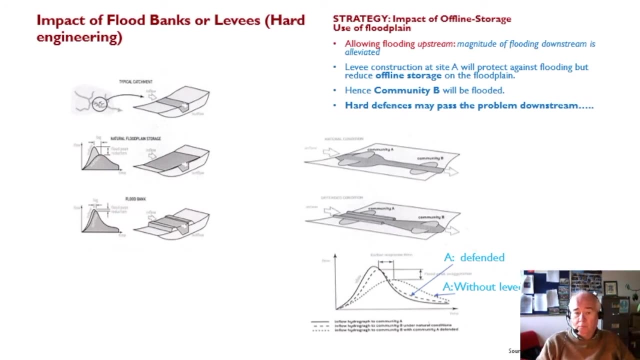 but the question is: are they the right answer for the future? here we can see recent flood defences in Keswick in the Lake District. The problem with defences such as levees is that, while they may do a good job locally in protecting a town or a community, 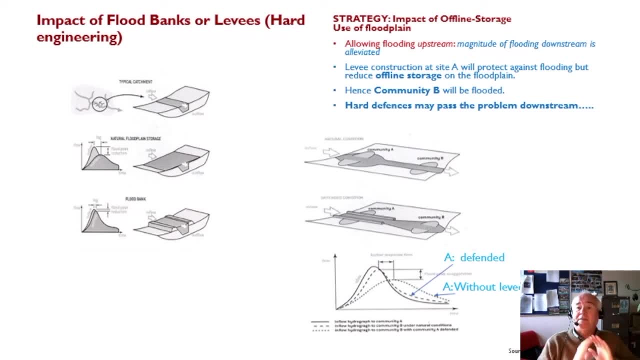 they keep the water in the river and so, in a sense, they pass the problem downstream, Allowing the river to flood, stores flood water on the floodplain, and that's what rivers do, naturally. That's what a floodplain's for: to store water. 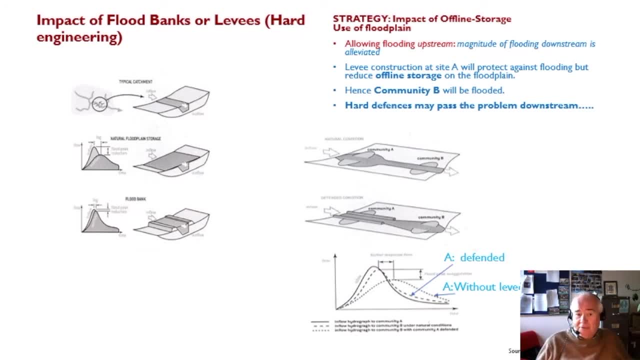 Rivers do that. It's natural. If you prevent flooding, you will send more water downstream. So if you have two communities and one is flooded and it's protected by levees, such as Community A here, then the likelihood of flooding at Community B. 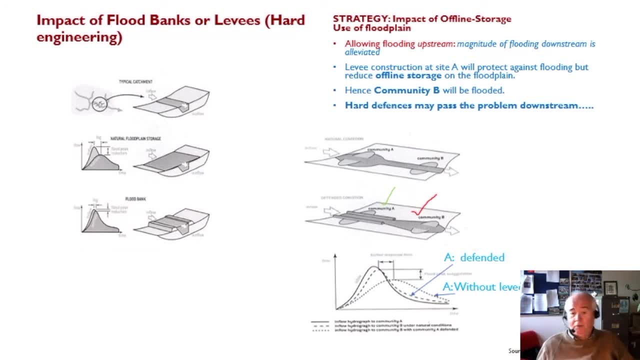 is increased. If you let flooding occur at Community A, the flooding likelihood at Community B is reduced. We can use that knowledge to try and store water in areas where it doesn't matter if flooding occurs, in order to protect downstream areas where flooding might have more serious consequences. 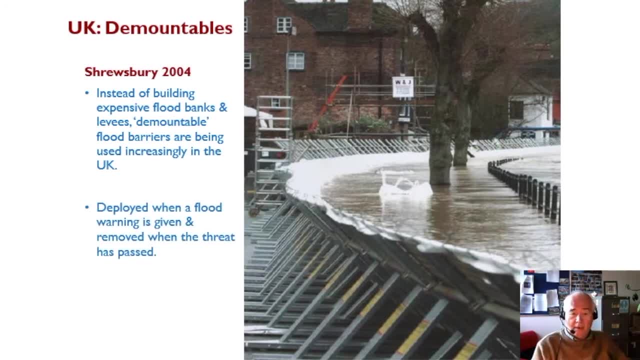 One evolution in flood management in recent years has been the development of portable levees or portable flood walls, and these are known as demountables, seen here in Sheffield. The advantage of those is that they protect the urban area against flooding, but that can then be removed. 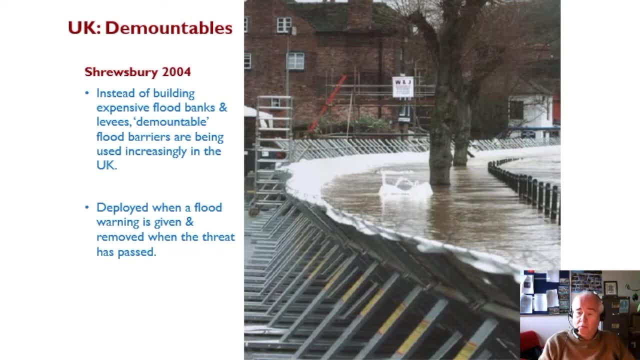 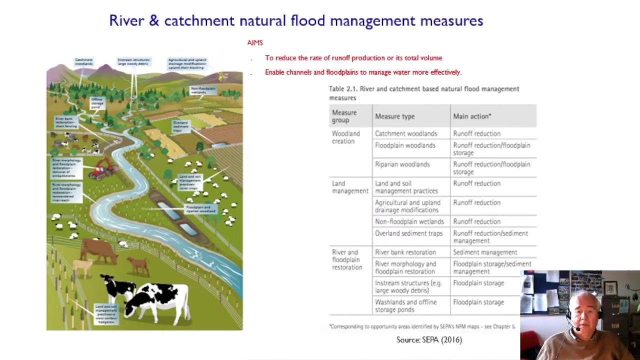 So they generally have less impact on the local landscape and on local ecology and wildlife than much bigger scale hard defences. Of course, they may not be so effective against extreme floods. however, An alternative to the hard engineering approach has been gaining ground. 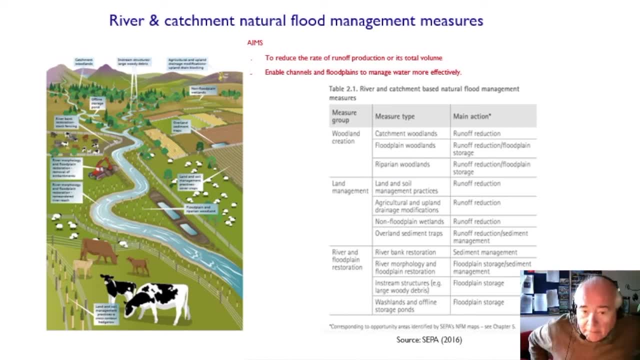 amongst flood managers really since the late 20th century. And this is the approach of flood abatement: It actually lets intervene in the hydrological cycle before the water gets into the rivers, in some cases by making the landscape better at storing rainfall, of absorbing rainfall. 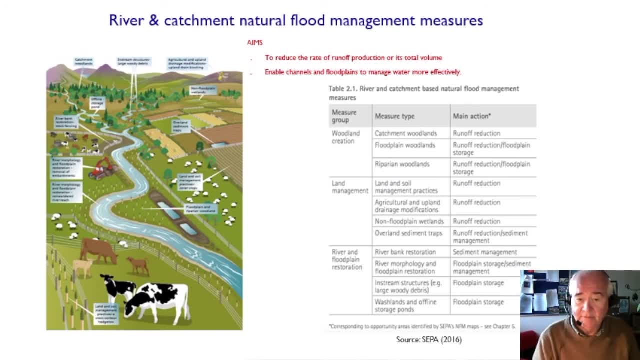 so that it doesn't travel from the catchment into the river. It also includes using natural floodplain to store water where that's not going to be a hazard. These measures, collectively known as flood abatement, involve rewilding catchment woodlands. 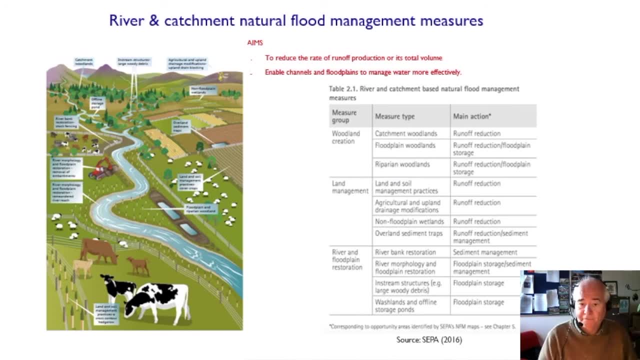 floodplain. woodlands to absorb runoff. managing the land and soil that we've already seen with respect to agricultural practice to encourage practices that absorb water rather than pass them into the river. The creation of wetlands or catchment sites. sediment traps to store material. 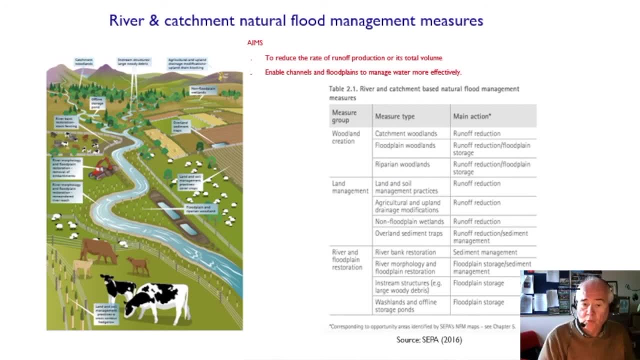 to prevent the rivers silting up and becoming more hazardous. The restoration of floodplains. and having structures within the upland parts of river catchments which store some of that runoff before it moves downstream to produce a flood hazard. All of these approaches are concerned with 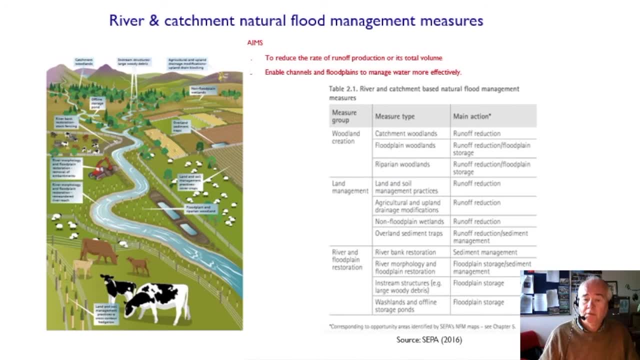 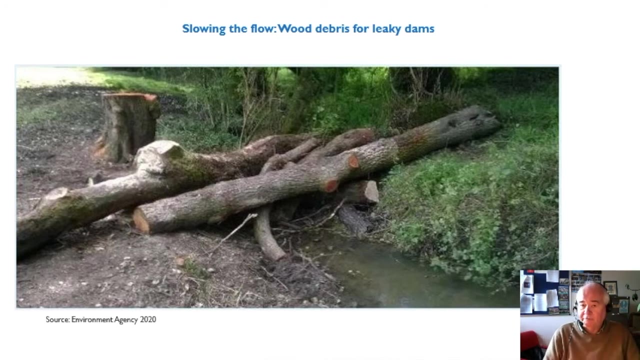 managing the flow before it becomes a hazard further down the river catchment. Perhaps some of these more environmentally friendly approaches to flood management have become more well known in recent years under the title or under the description of slowing the flow. The idea is to keep the water. 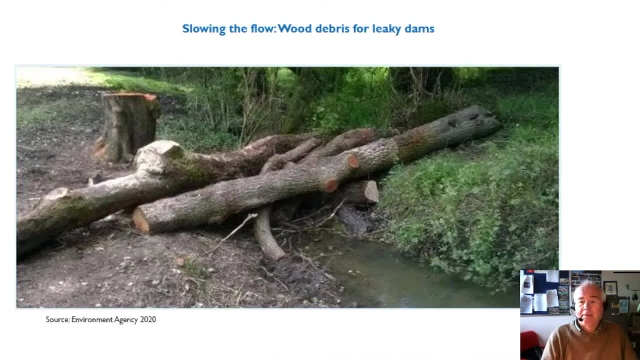 from getting from the headwaters of the river into the channel downstream. We can use this. rather than building concrete or hard engineering structures, we can use natural materials, Such as here. we can see the use of natural woody debris. This is an example of a leaky dam. 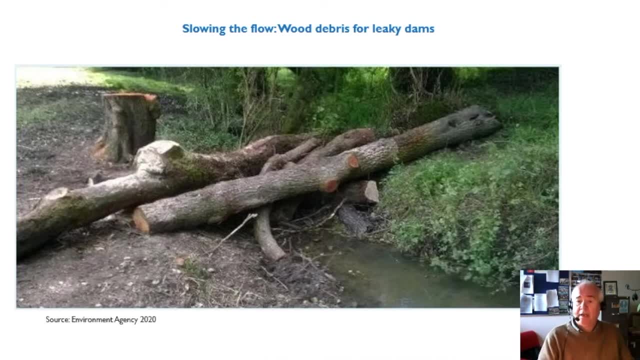 And these can be put in the headwaters, the head streams of the river network. And what they do is when it rains heavily and runoff starts to occur- is they pond that water and just delay it. The water spills out of it, It goes onto the land surface. 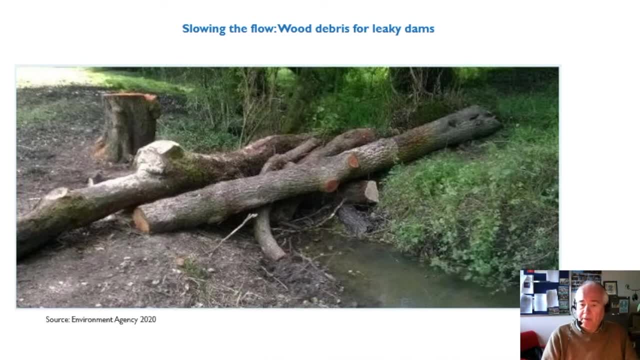 and is absorbed by the soil. So the role here is not only to reduce the amount of water moving downstream, but the critical element is delaying it, Because if you can spread out the arrival of water from upstream, you will generally reduce the peak of the flood hydrograph. 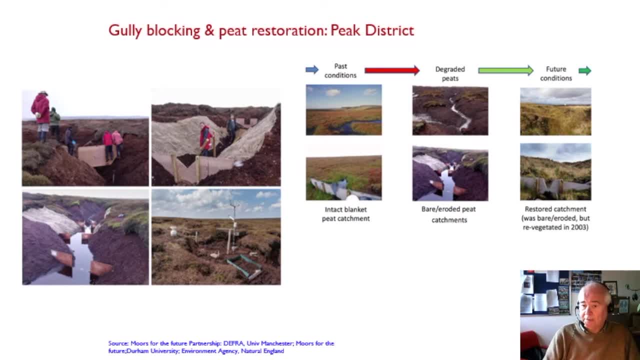 Other examples of slowing the flow include peat restoration in the highlands of Britain. These include simple mechanical structures such as small dams using wood material or natural materials, Particularly where the peat has become eroded, such as these peat grafts in the peat district. 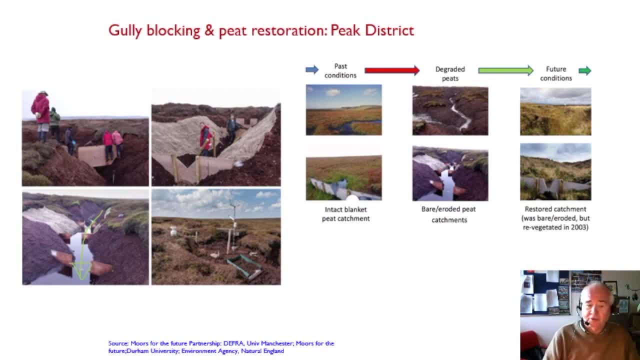 These eroded features, where the vegetation has been lost, channel the water and mean that it runs off of the peat district highlands very quickly into the local rivers, And that exacerbates flood hazard If you can retain that water by small gully blocks. 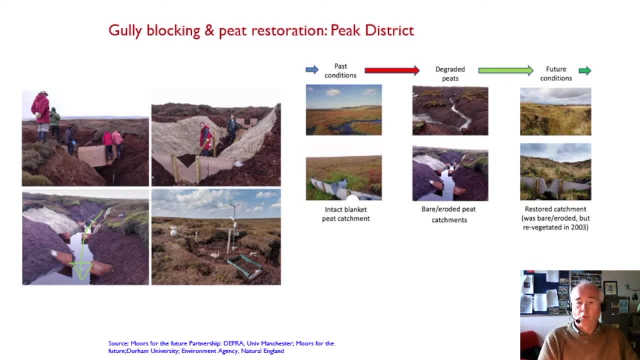 as they're called again. that keeps the water back, Delays it, Reduces the peak of flow downstream. But that's not all. There's a major conservation issue Here: restoring the peatland vegetation, The production of healthy peat. 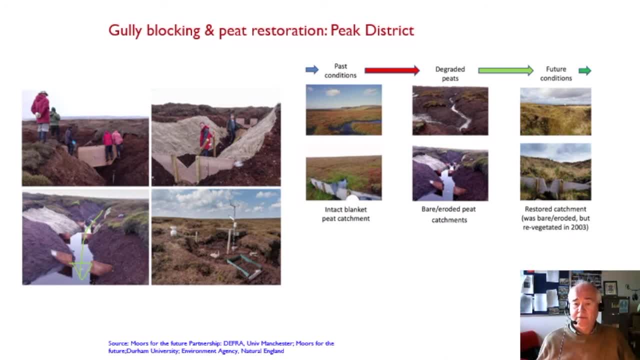 More vegetated land surfaces. Retain what runoff there is, Slow it down, Absorb it. So a combination of restored vegetation and simple slowing the flow structures aims to reduce the rate at which water gets from the highlands into some of these steep northern rivers. 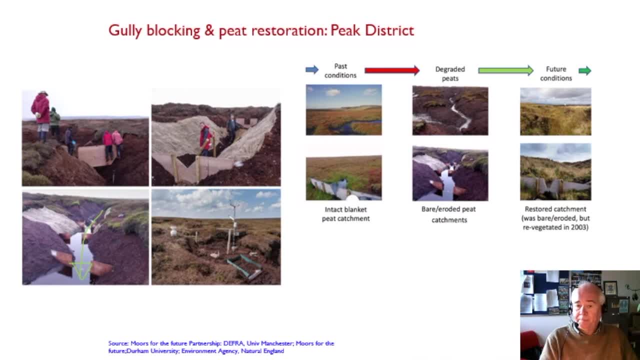 to reduce the intensity of flooding. The results from these types of study and these types of projects so far are not conclusive, But there certainly is evidence that certainly for the smaller floods and the more frequent flood events, they are reducing the intensity of the floods. 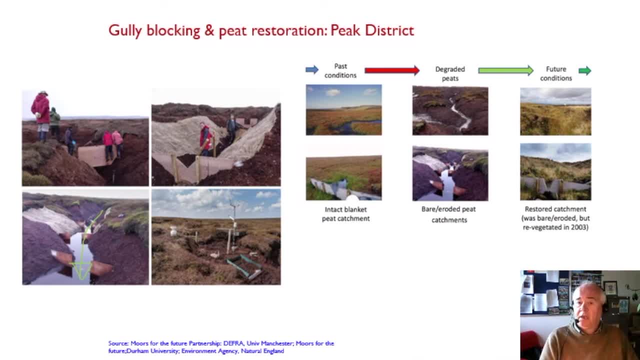 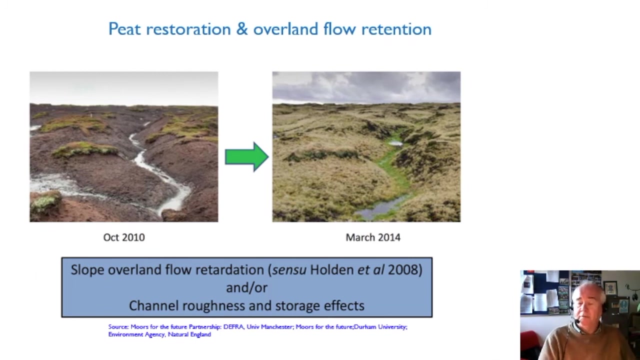 The big question for flood research is whether these types of more natural interventions will have an effect upon the extreme flood events that may become more common In an energised atmospheric system. But there's certainly hope, And not only is it about reducing the frequency of floods. 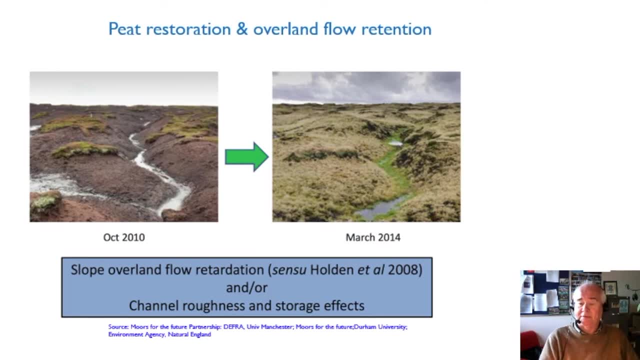 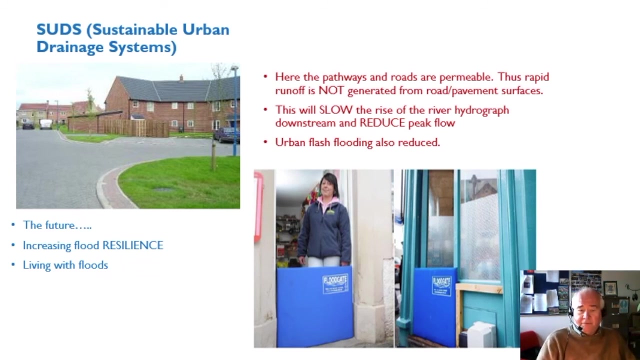 but it's also about creating a healthy landscape in which the natural processes of water retention and flood control can be used, rather than the ecologically damaging hard engineering approaches that we've been more used to in recent years, These types of approach of slowing the flow. 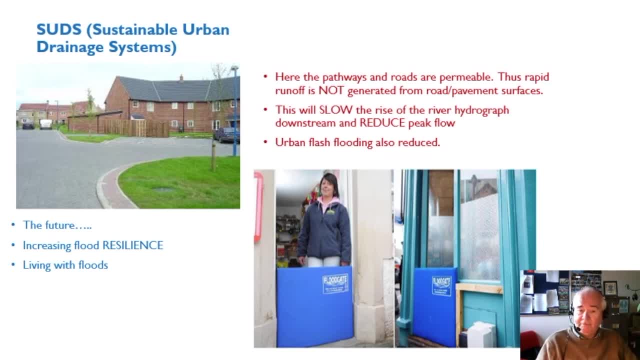 are not only used in natural environments, but can be used in towns and cities. They generally go under the name of SUDs or Sustainable Urban Drainage Systems. The idea here is to build permeable roads, to have green roofs on housing estates or roughened roofs. 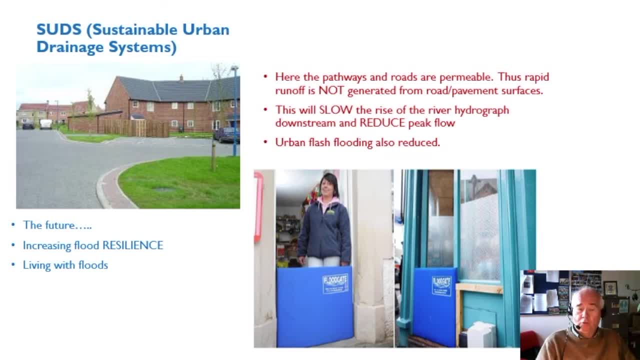 to slow down the rate at which water transfers from the roofs and from the roads and runs off. It involves local sinkaways with vegetation and trees to collect the runoff from local housing estates, store it and preventing it getting into the rivers rapidly. So this slowing the flow concept. 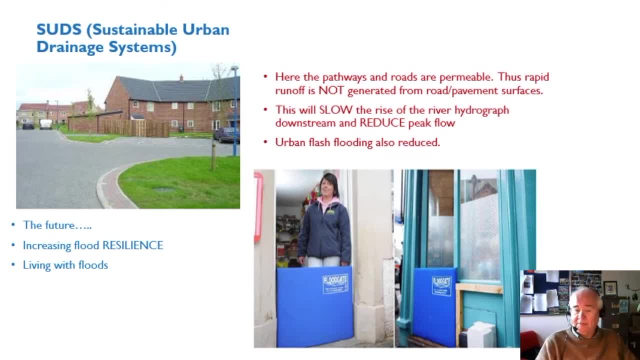 can occur in cities as well as in the countryside. Another approach is to start thinking about living with floods In an energised hydrological system in a globally warmed world. even if we take the measures that we hope will come out of COP26, we're still likely to see. 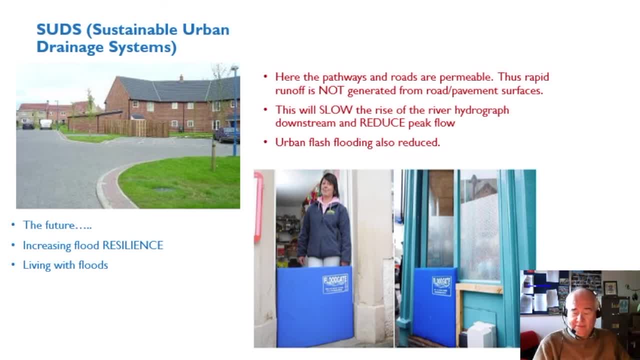 increased winter precipitation and increased flood hazard. So perhaps we should start thinking about living with floods rather than living with floods. So perhaps we also start to think about living with floods becoming resilient, recovering more quickly from flood events, but also preventing them at the household level. 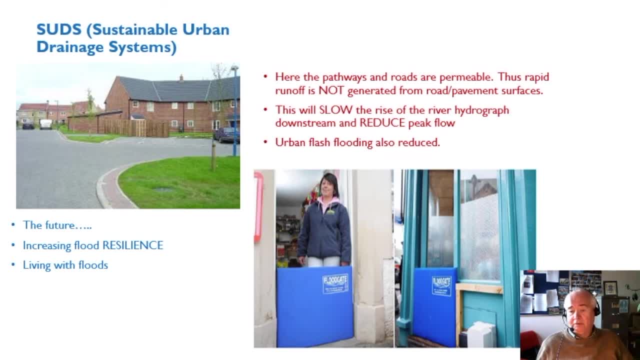 So the use of resilience measures such as the flood gates and the flood doors used on individual shops and houses will help us to learn to live with flooding, to learn to accept it as part of the world in which we live, rather than constantly fighting against it. 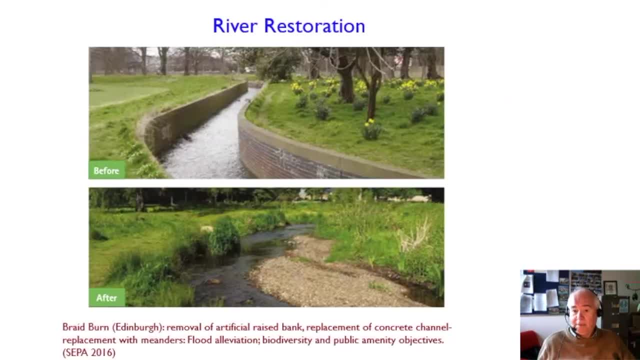 That's a view for discussion and debate. Perhaps the biggest development in flood management in the last 50 years, however, has been the move to river restoration, That it may be beneficial to rip out and take out some of the engineering that has made our rivers. 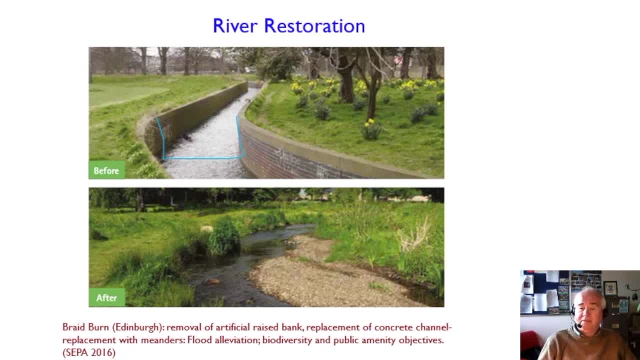 into boxes devoid of wildlife, Efficient perhaps at preventing flooding- but then that's becoming open to question- but actually damaging to our environment. Returning rivers to their natural state: this is the river restoration movement that's becoming a bigger part of flood control policy in the 21st century. 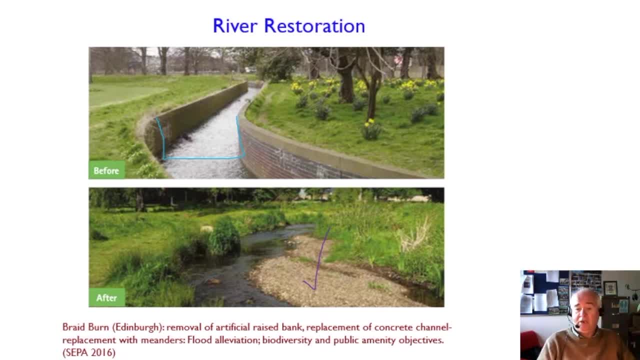 Restoring the link between the river channel and the flood plain. Letting rivers flood, because that's what they're meant to do, But trying to encourage that flooding to occur in areas that won't be harmful or hazardous, That has the impact of restoring.